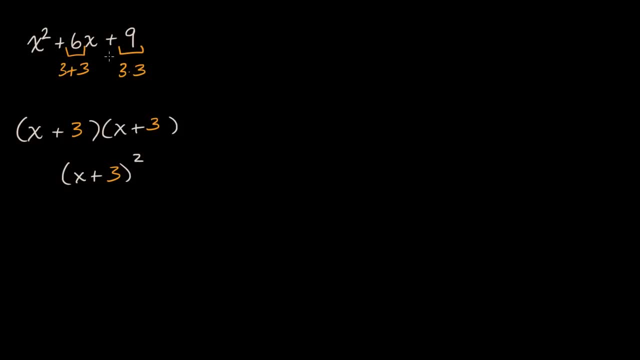 that made us recognize- or maybe now we will start to recognize- as it being a perfect square. Well, I have, of course, some variable that is being squared, which we need. I have some perfect square as the constant and that whatever is being squared there. 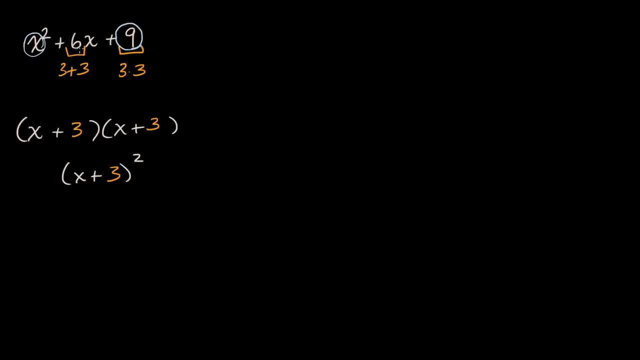 I have two times. that is the coefficient on this first degree term here. Let's see if that is generally true And I'll switch up the variables just to show that we can. So let's say that I have a squared plus 14a. 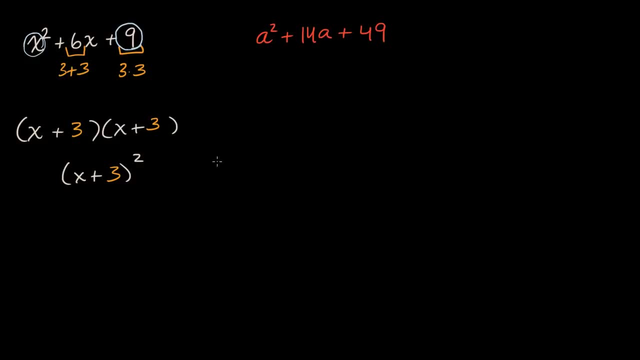 plus 49.. So a few interesting things are happening here. All right, I have my variable squared. I have a perfect square constant term that is seven, squared right over here, And my coefficient on my first degree term here. that is two times the thing that's being squared right. 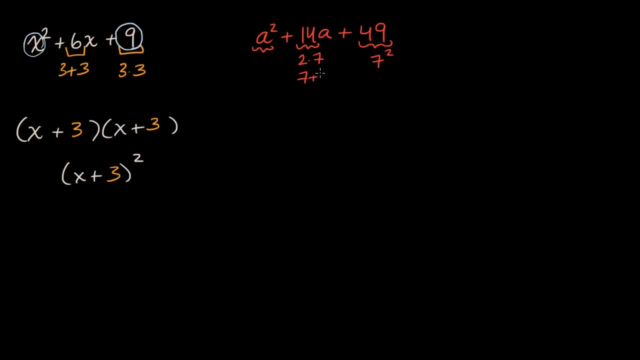 That is two times seven, or you could say it's seven plus seven. So you can immediately say: okay, if I want to factor this, this is going to be a plus seven squared, And you can of course verify that by multiplying out. 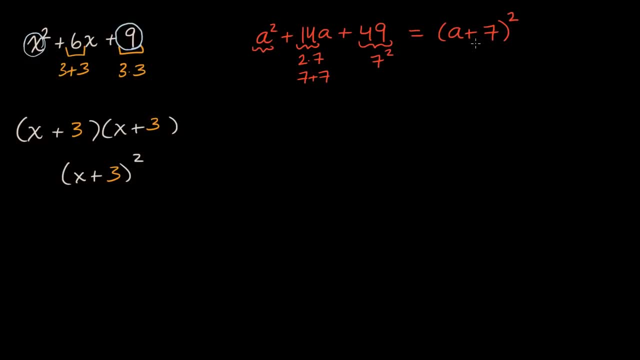 by figuring out what a plus seven squared is. Sometimes, when you're first learning, it's like, hey, isn't that just a squared plus seven squared? No, remember, this is the same thing as a plus seven times a plus seven. 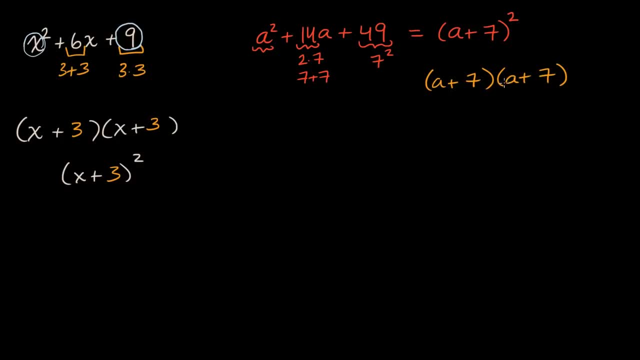 And you can calculate this by using the FOIL F-O-I-L technique. I don't like that so much because you're not thinking mathematically about what's happening. Really, you just have to do the distributive property twice here. 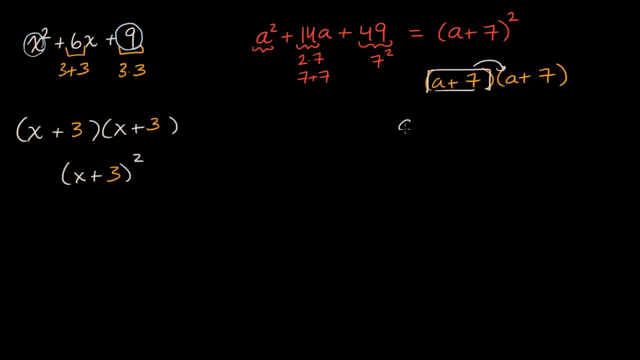 First you can multiply a plus seven times a, So a plus seven times a. And then multiply a plus seven times seven, So plus a plus seven times seven, And so this is going to be a squared plus seven a plus. now we distribute this seven plus seven. 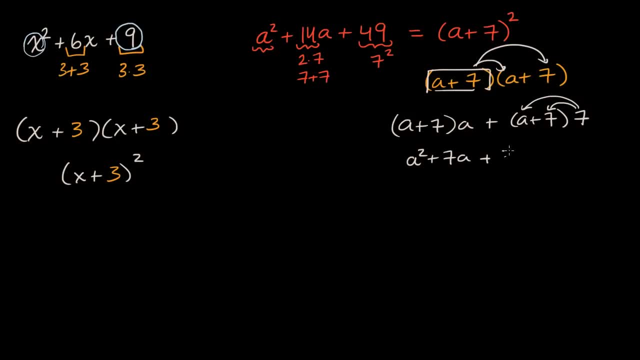 So this is going to be a squared plus seven a plus. now we distribute this: seven plus seven a plus 49.. So now you see where that 14a came from. It's from the seven a plus the seven a. 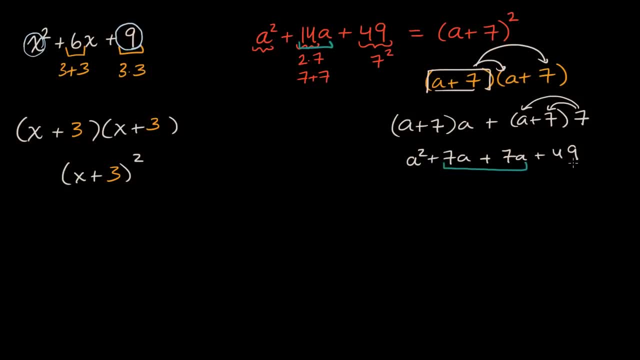 You see where the a squared came from And you see where the 49 came from, And you can speak of this in more general terms. If I wanted to just take the expression a plus b and square it, that's just a plus b. 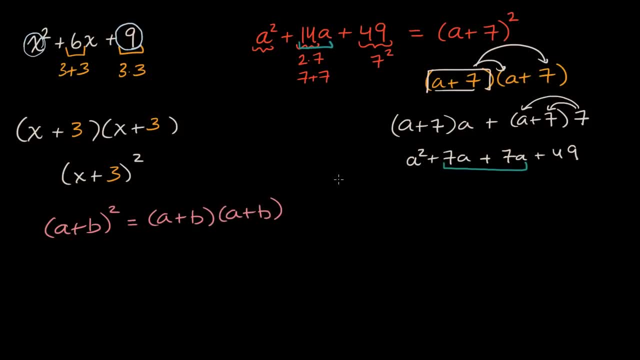 times a plus b, And we do exactly what we did just here. but here I'm just doing in very general terms with a or b, And you can think of a as either a constant number or even a variable, And so this is going to be if we distribute this. 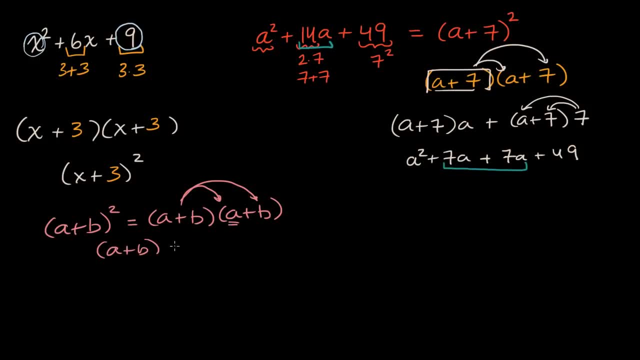 it's going to be a plus b times that a plus a plus b times that b, And so this is going to be a squared. now I'm just doing the distributive property again: a squared plus ab times b Plus ab plus b squared. 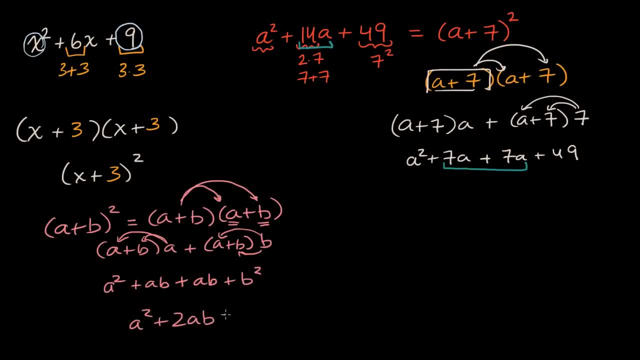 So it's a squared plus two, ab plus b, b squared. So this is going to be the general form. So if a is the variable which was x or a in this case, then it's just going to be whatever squared in the constant term is going to be two times that. 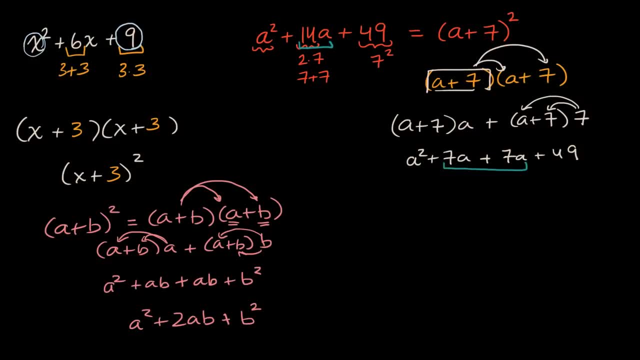 times the variable, So that there's some variation that you can entertain here. So if you were to see 25 plus 10x plus x squared and someone said, hey, why don't you factor that? Well, you could say: look this right here. 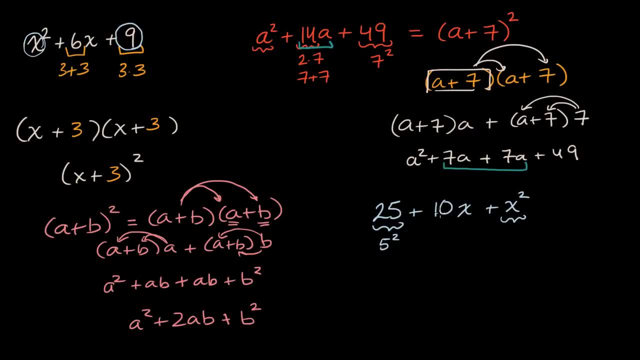 is a perfect square. it's five squared. I have the variable squared right over here. And then this coefficient on our first degree term is two times five, And so you might immediately recognize this as five plus x squared. Now, of course, you could just rewrite this polynomial: 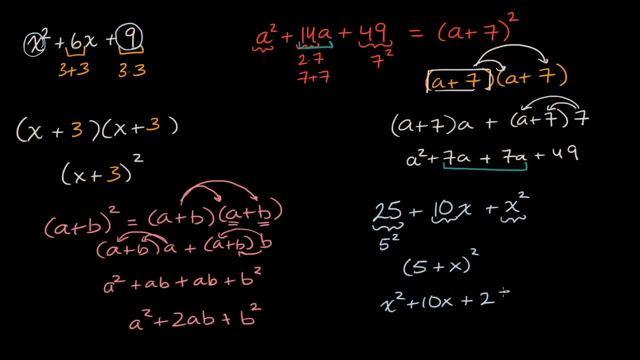 as x squared plus 10x plus 25.. In which case you might say: hey, okay, variable squared some number squared five squared two times that number is the coefficient here, So that's going to be x plus five squared. 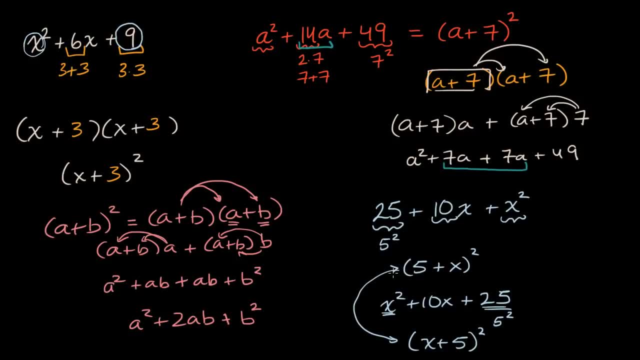 And that's good, because these two things are absolutely equivalent.